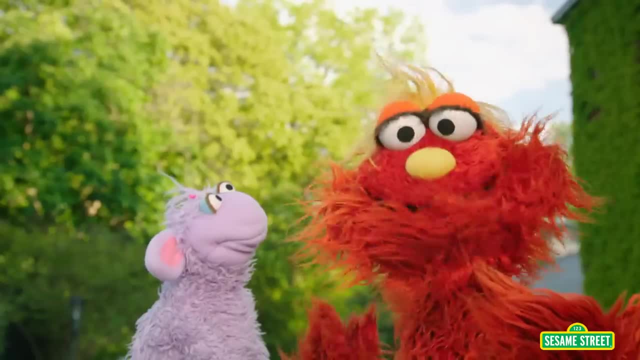 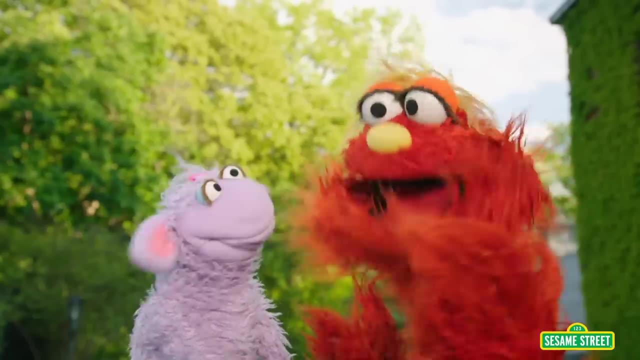 Ovejita. Hola, Murray Ovejita. what present can I make my mommy for her birthday? No se, Oh, you don't know, But you said you knew what to make her. Yo conozco a alguien que te puede ayudar. 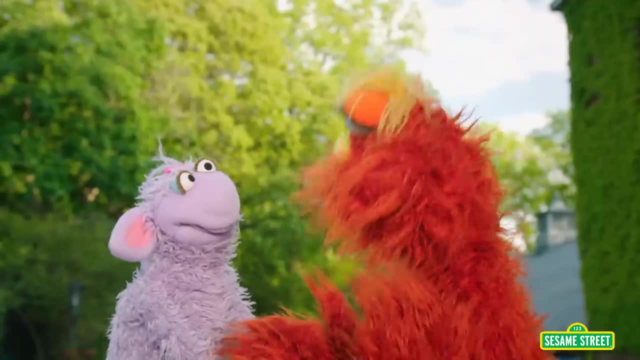 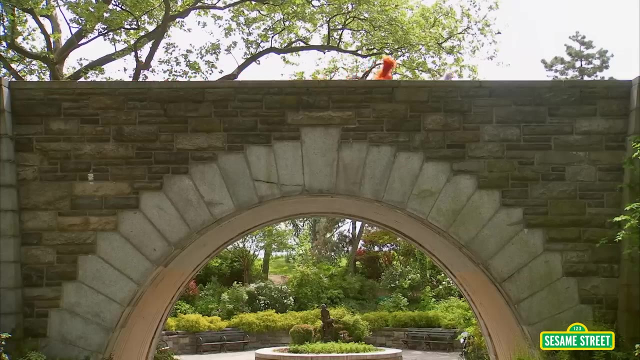 You know someone who can help me make a present? Uh-uh Who who Sigueme? Follow my little lamb. Murray has a little lamb. Murray has a little lamb who wears a little bow. Go, Murray, Together, they go everywhere. 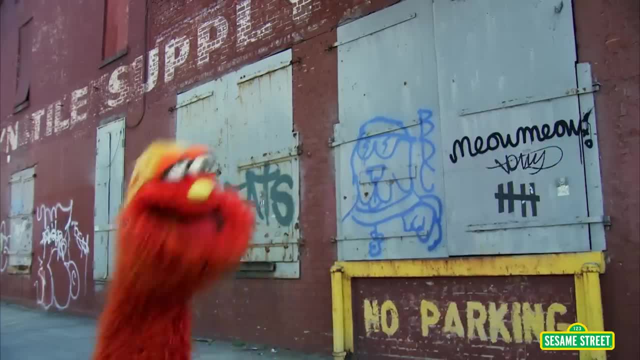 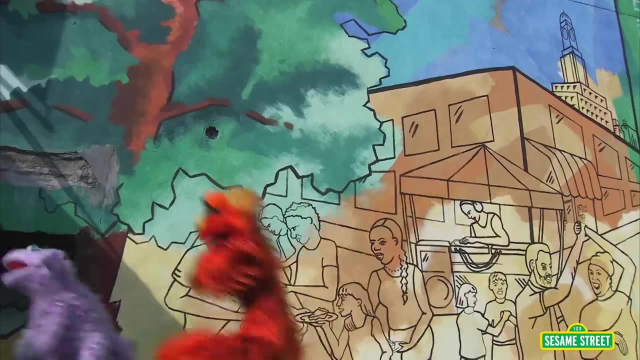 Amigos like to go Murray. He follows her to school Each day. they run, They spin, They strum, They spin. Hello, Murray. Yo, everybody loves to see a monster and his sheep And they all say Murray has a little lamb. 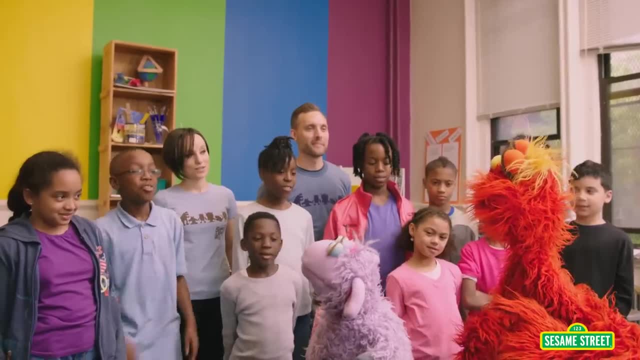 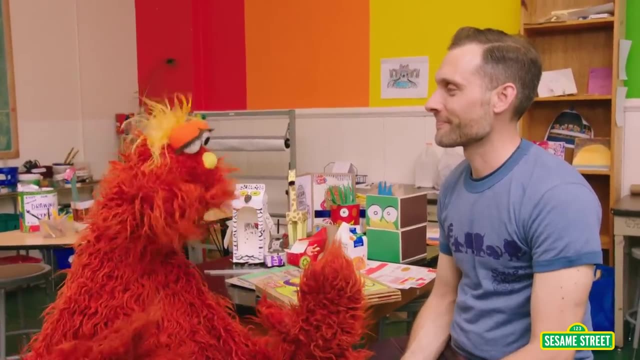 Oh, hey you guys. What school is this Recycled Art School? Oh boy, Hey Brian, Hey Murray, I have a question for you. OK, what I'm trying to think, what I can make my mom for her birthday. 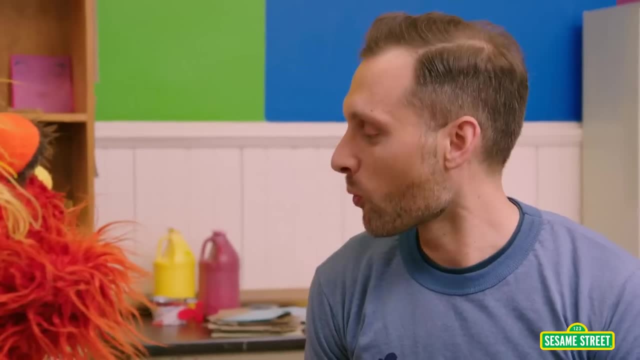 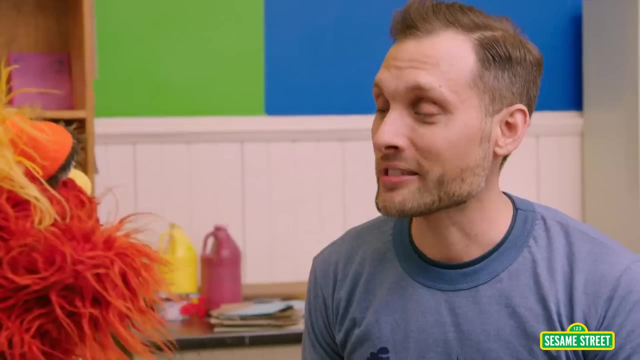 And I just don't have any ideas. Do you think you could help me? Well, we're going to use recycled materials to make some presents. Excuse me, Brian, What does it mean to recycle? Recycle means when you reuse something. 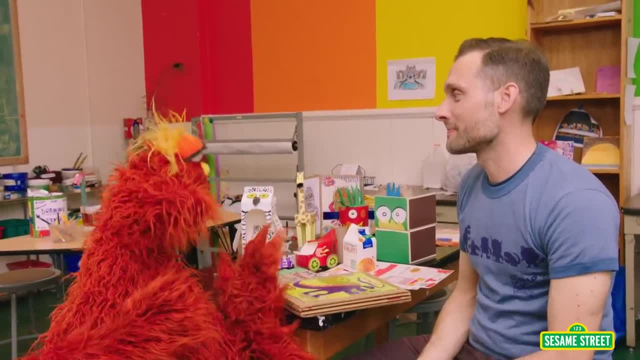 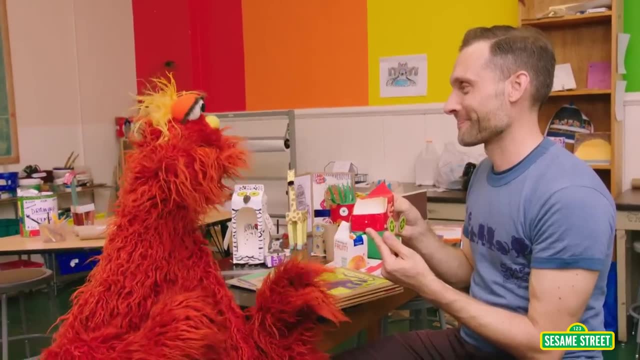 instead of throwing it away. Really Well, what kind of things can you make here out of recycled things? What do you think of this, this car? I think that car is awesome. Where did you buy it? I didn't buy it. 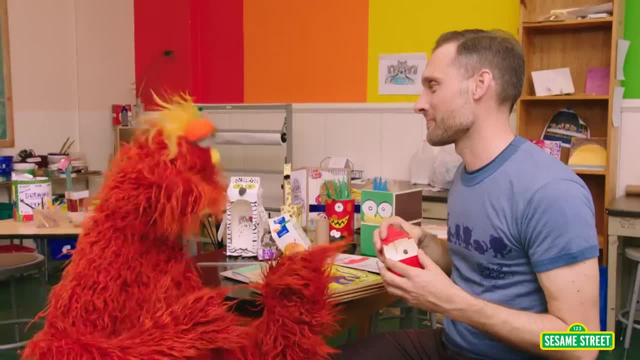 I made it, You made that car. I did: yeah, Wait, I can make something like that cool car. You can. yeah, Whoa, whoa. Well, my mom's not really into cars. What other stuff can we make? 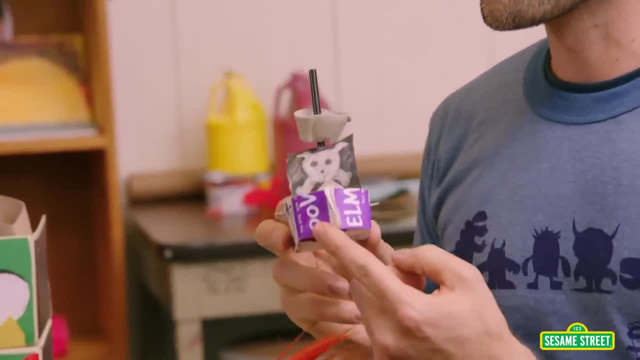 All right, let's see what else we have. Does she like boats? She likes to go out, She likes to go on cruises. so maybe she would like a boat. But you know what I just remembered? Sometimes mom gets seasick. 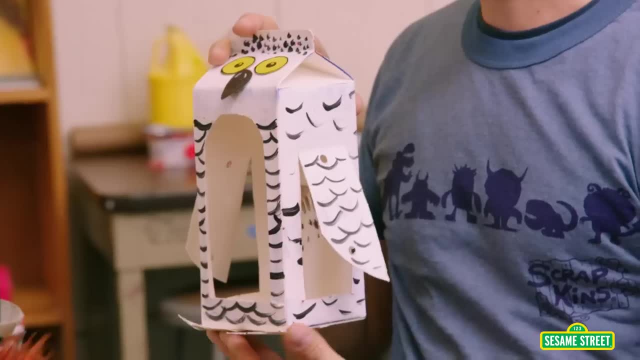 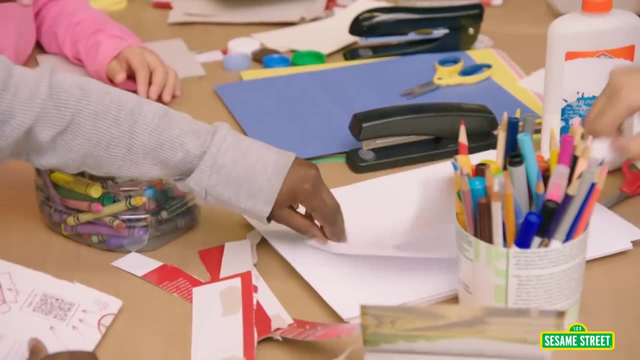 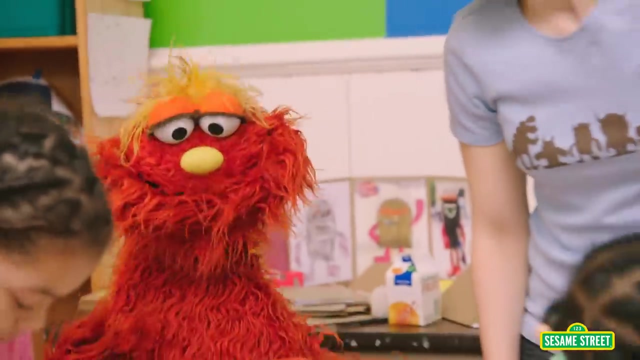 What else you got? OK, let's see A bird feeder. Hmm, so many choices. Oh, I'm going to need some time to think: Hey, you guys, What are you working on at this table? What are you making? 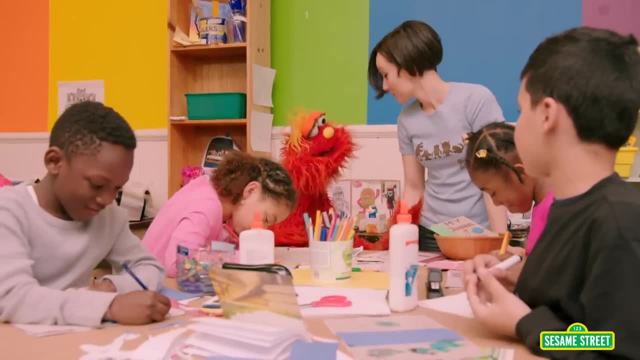 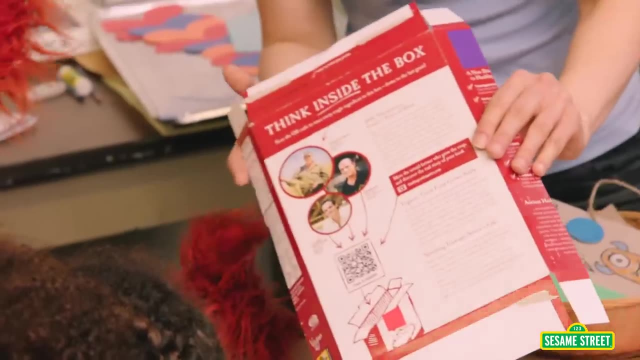 Journals, Journals. Candace, how do you make journals out of recycled material? Well, Murray, we're making these out of cereal boxes, Cereal boxes. You take a cereal box, fold it in half and then it makes a book like this: 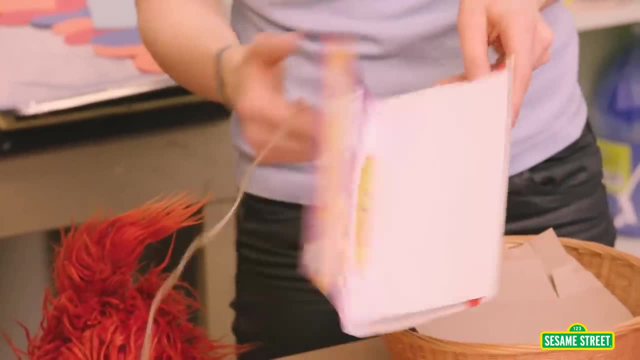 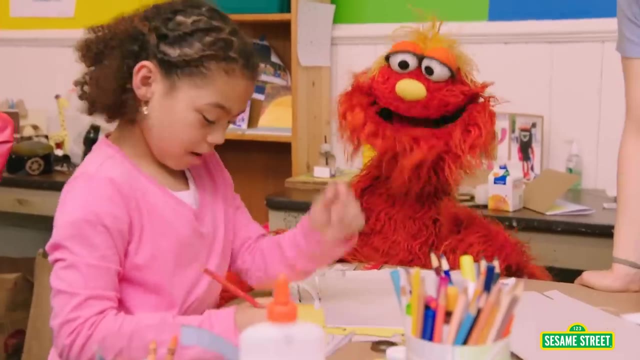 Whoa, and then you put paper in there, All the paper you need, And then you wrap it closed. That is so cool, Whoa. No one can get in there. Damari, what's on your journal? Soccer, Whoa. 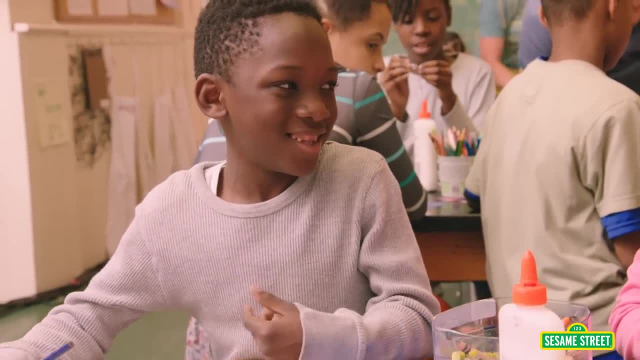 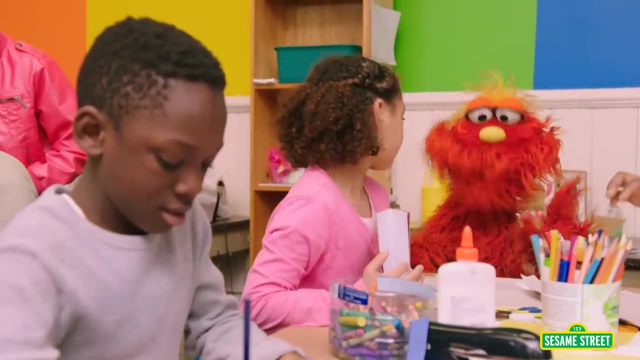 Who are you making your journal for? Damari, My mom. Your signature It's a gift for your mom. Hmm, Maybe I should make a journal for my mom, But I haven't decided yet. I'm going to see what they're making over there. 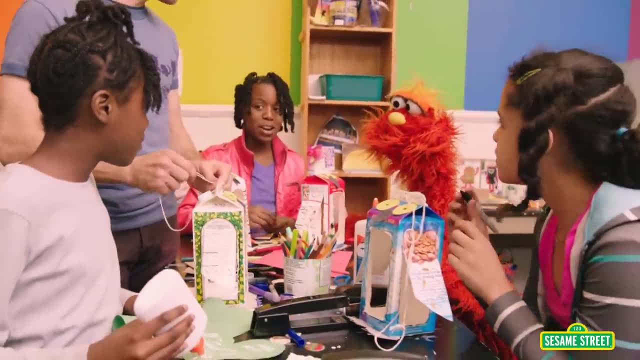 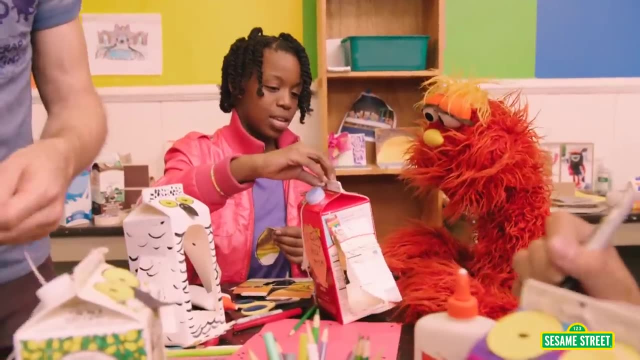 Hey guys, What are you making at this table? Bird feeders, Bird feeders. Whoa, Hey Daniela, what kind of bird feeder are you making here? It's an owl. Cool, can I see it? Let me see. 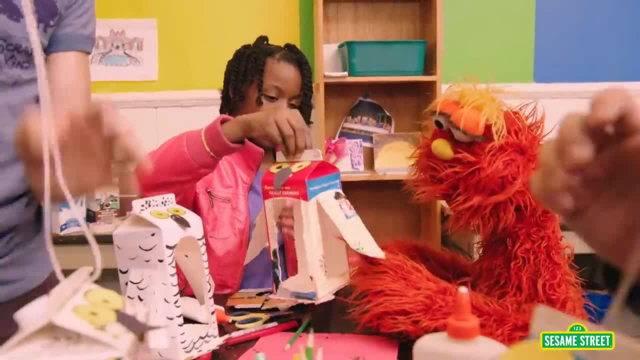 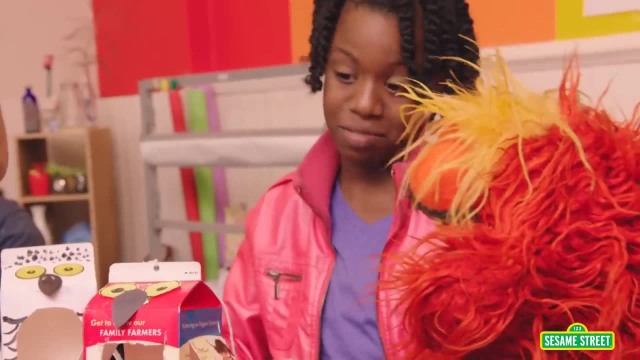 Whoa, it looks like an owl. And how did you make it? I made it by using recycled materials: Milk carton, Yeah, Cardboard, Right, And that's it. That's very cool. And who are you making your bird feeder for? 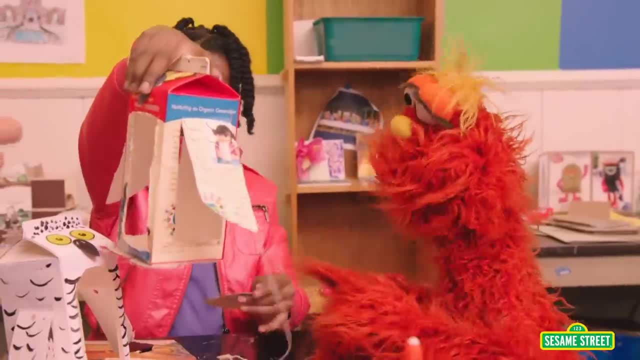 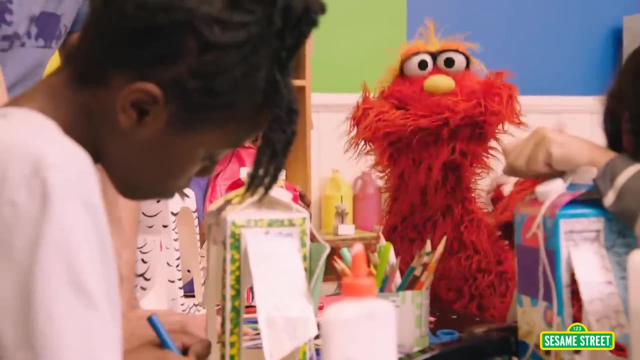 Mom. It says I love my mom. That is a nice gift, Thank you. Hmm, Maybe a bird feeder, But I'm not sure yet. Let's see what else I can make. Hey, what are you guys making? Tube monsters. 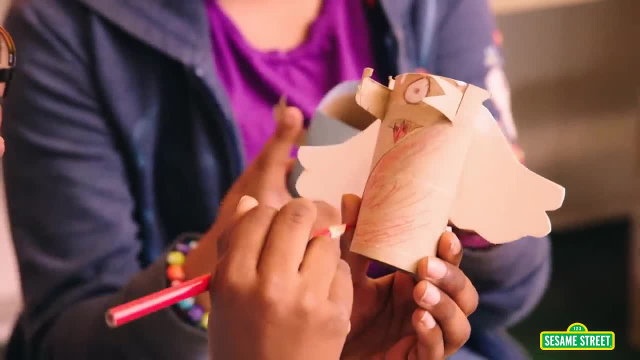 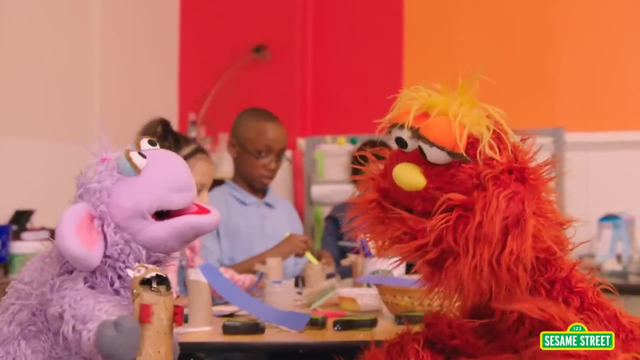 Oh, oh, oh oh. Tube monsters. My mom's a monster, That's it. I'm going to make a tube monster for my mommy out of this toilet paper tube. OK, Brian, how do we make it? All right, everybody. 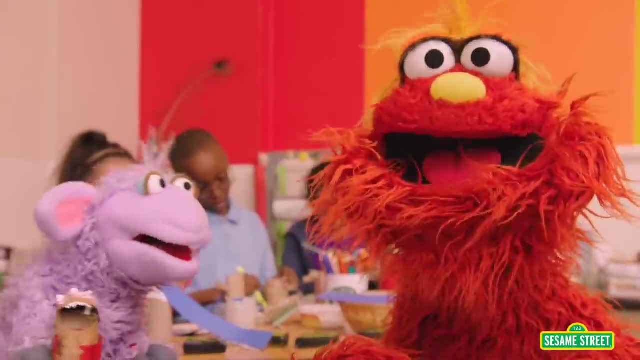 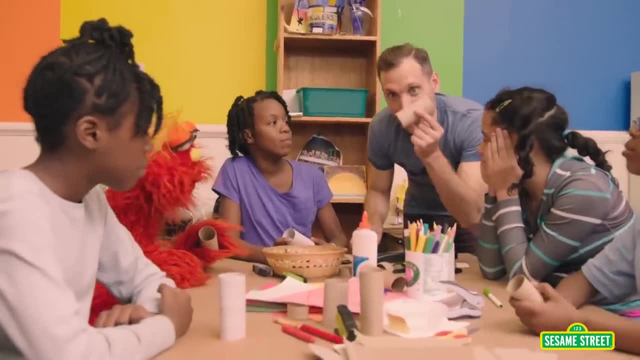 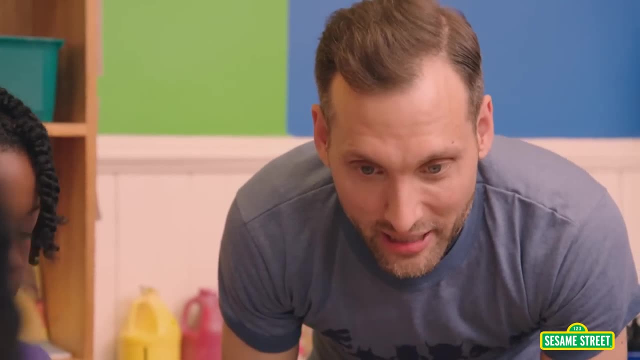